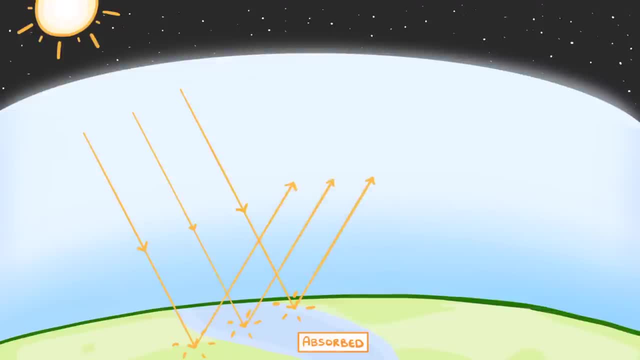 is either re-emitted or reflected back into the atmosphere towards space. Although some of this radiation does make it back to space, most of it actually hits particles of gas in our atmosphere, which will absorb all of the energy, And after a short delay, the particles then re-emit the 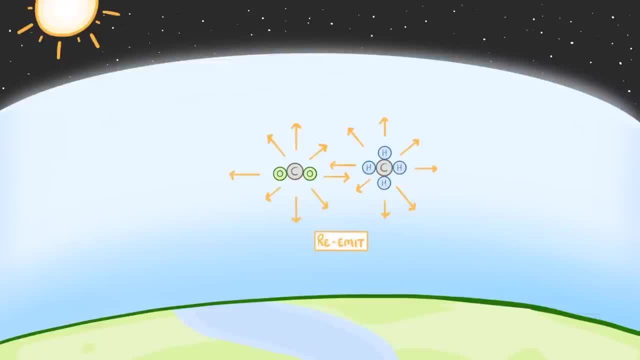 energy in random directions. This means that some of the energy will be re-emitted towards space and some towards the Earth. Either way, though, just like before, most of the energy will collide with another gas particle before it can leave the atmosphere. This process of being absorbed and re-emitted by gas particles happens over and over again. 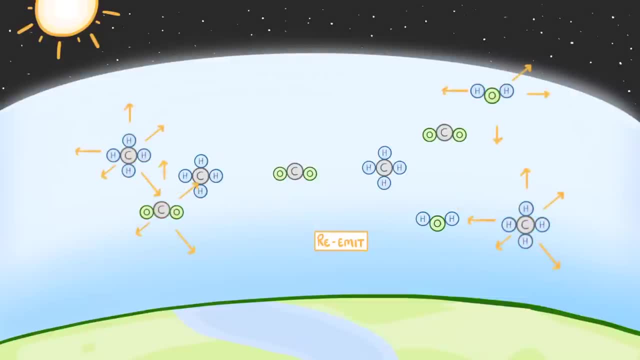 which means that the heat energy stays close to Earth far longer than if there was no atmosphere, And it's this process that keeps the Earth at a warm and stable temperature. As you can see in this picture, this process happens with lots of different molecules. 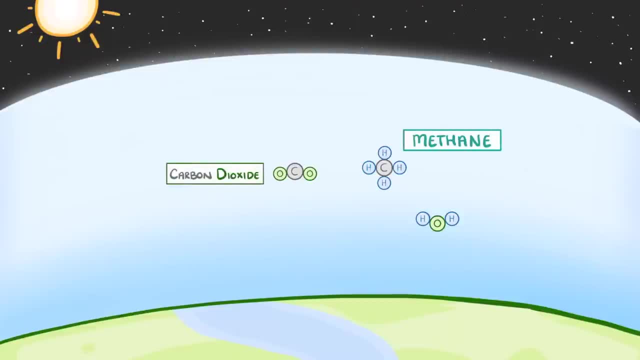 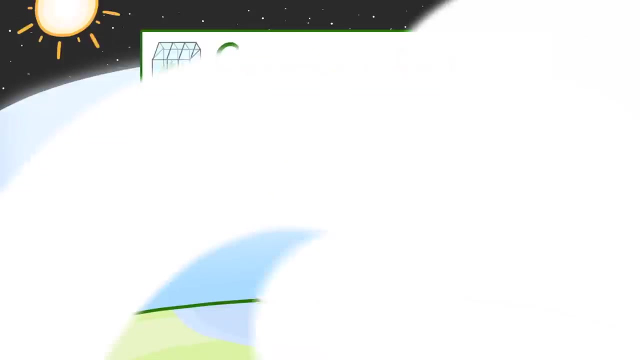 including carbon dioxide and methane, but also water vapor. We call this group of gases greenhouse gases, and although the greenhouse effect that they cause is essential for life, it's also responsible for global warming In the 4.5 billion years that the Earth has been around. the strength of this greenhouse. 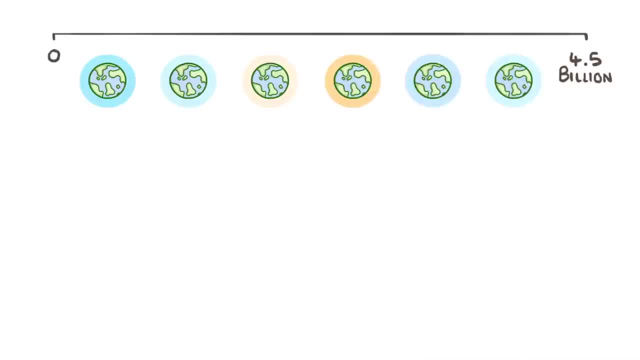 effect has grown and shrunk over and over, And this is happening again right now, mostly due to humans releasing loads of carbon dioxide and methane into the atmosphere. The problem is that, as these gases accumulate and the greenhouse effect gets stronger, the Earth warms up, which we call global warming. 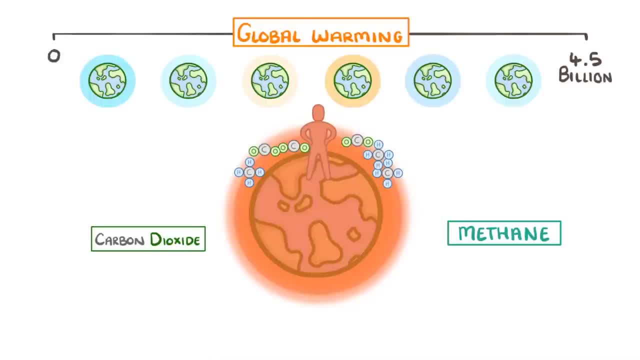 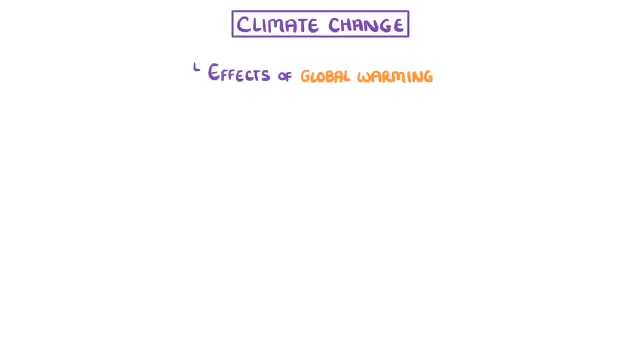 In the past 100 years, our planet has already got almost a whole degree warmer, and it's on track to rise a lot more if we don't do something major to stop it. Now the term climate change is a bit different. It's more about the effects of this global warming. 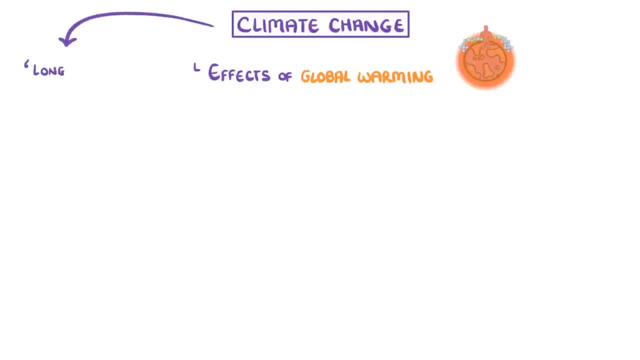 on the climate And remember. climate, as David said, just describes long-term weather patterns. For example, one of the consequences of global warming is that rare weather events like droughts, hurricanes and floods will become both more common and more severe.